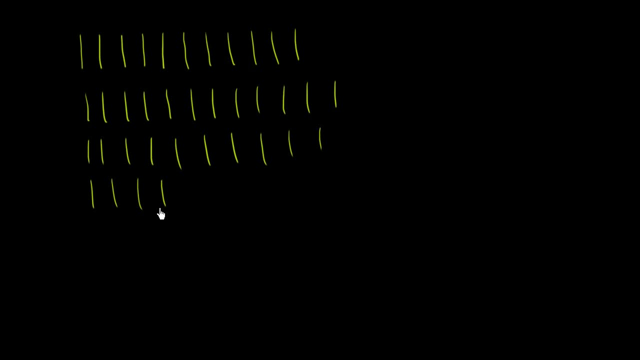 to represent whatever number this is. So first of all, let's just think about what number this actually is: One, two, three, four, five, six, seven, eight, nine, 10,, 11,, 12,, 13,, 14,, 15,, 16,, 17,, 18,. 19,, 20,, 21,, 22,, 23,, 24,, 25,, 26,, 27,, 28,, 29,, 30.. 31,, 32,, 33,, 34,, 35,, 36,, 37.. 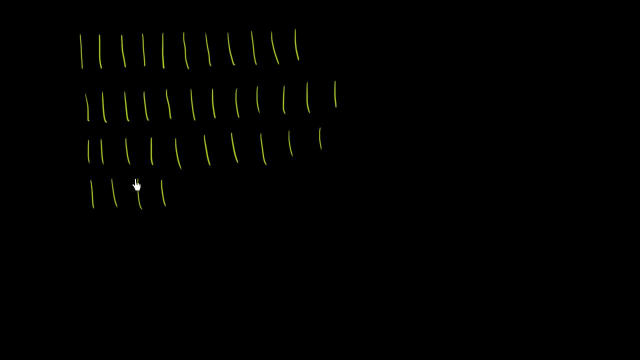 So you wish that there was a better way to represent this number, which we now call 37. And maybe when you were first trying you might not have even called it something called 37. You would just call it this number this number of days since my birthday. 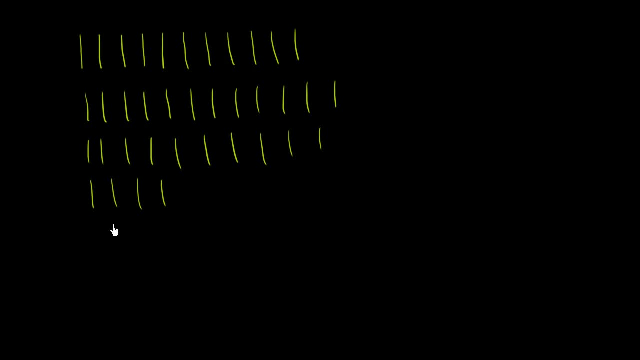 And say: well, look, what if there was an easy way to group the numbers? You know I have 10 fingers on my hands. What if I were to group them into tens, And then I would just say how many groups of 10 I have. 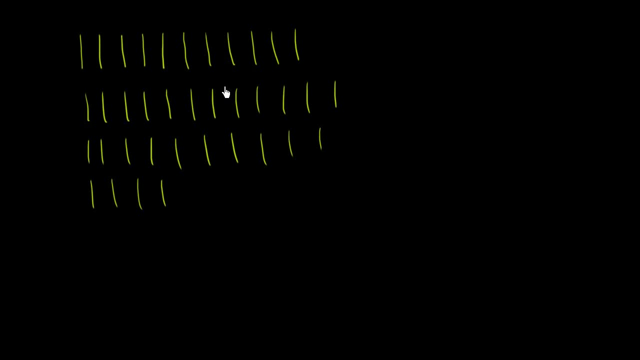 and then, how many ones do I have left over? Maybe that would be an easier way to represent this quantity here, And so let's do that. So one, two, three, four, five, six, seven, eight, nine, 10.. 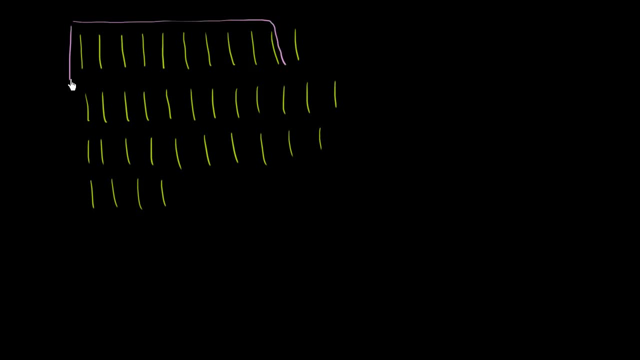 So that's a group of 10 right over there. And then you have one, two, three, four, five, six, seven, eight, nine, 10.. So this is another group of 10 right over here. And then let's see: 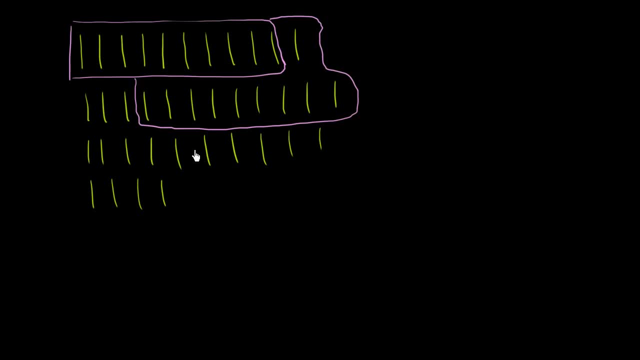 We have one, two, three, four, five, six, seven, eight, nine, 10.. So that is another group of 10 right over there. And then finally you have one, two, three, four, five, six, seven. 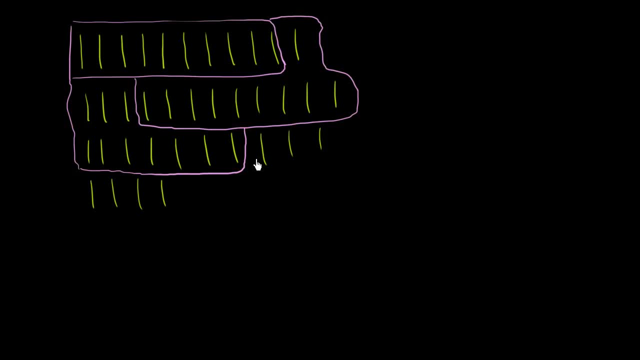 So you don't get a whole group of 10, so you don't circle them. So just by doing this very simple thing now, all of a sudden, it's much easier to realize how many days have passed. You don't have to count everything. 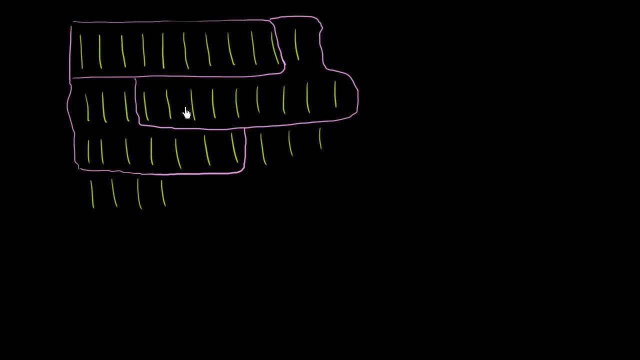 You just have to say, okay, one group of 10,, two groups of 10,, three groups of 10.. Or you could say one, two, three, 10s, And so that's essentially 30. And then I have another one, two, three. 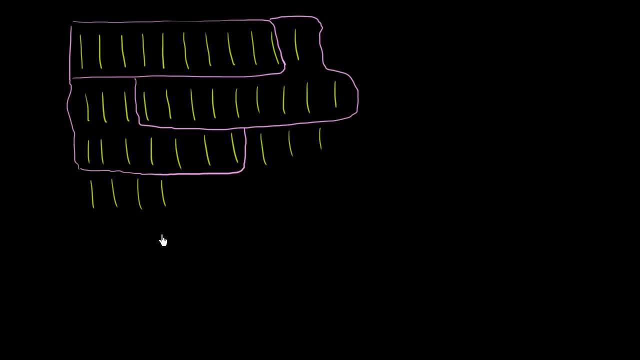 four, five, six, seven, And so you say: oh, I have 30 and then seven, If you knew to use those words which we now use, And this is essentially what our number system does, using the 10 digits we know of. 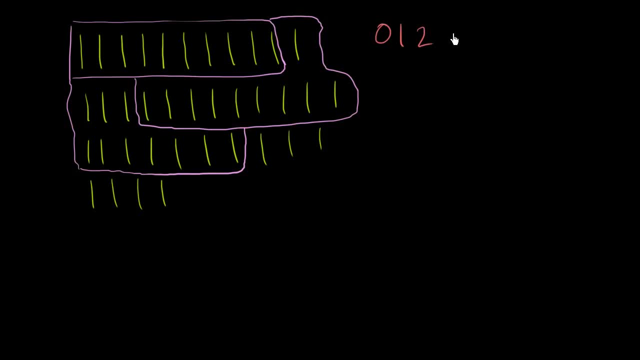 The 10 digits we know of are just zero, one, two, three, four, five, six, seven, eight, nine, And what our number system allows us to do is, using only these 10 digits, we can essentially represent any number we want. 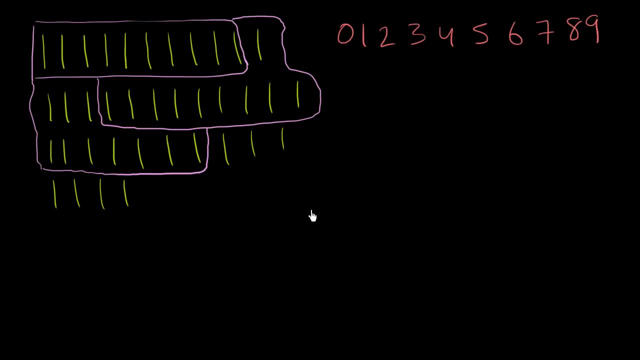 in a very quick way, a very easy way for our brains to understand it. So here, if we want to represent three 10s, we would have put a three in what we would call the 10s place. We would put a three in the 10s place. 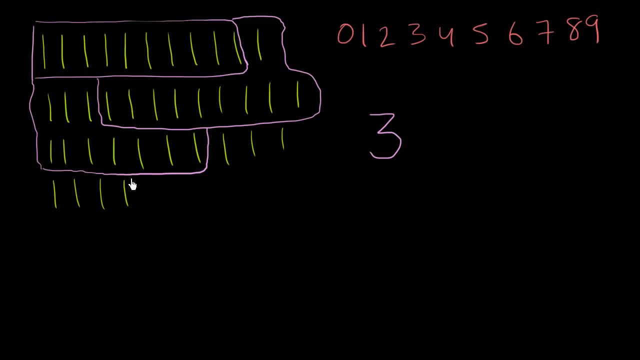 And then we would put the ones one, two, three, four, five, six, seven. We'd put the seven in the ones place. And so how do you know which place is which? Well, the first place, starting from the right. 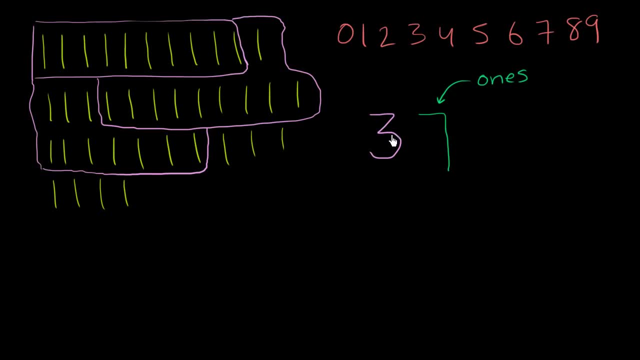 the first place is the ones place, And then you go one space to the left of it, you get to the 10s place And, as we'll see, you go one more space. you go to the hundreds place, But we'll cover that in a future video. 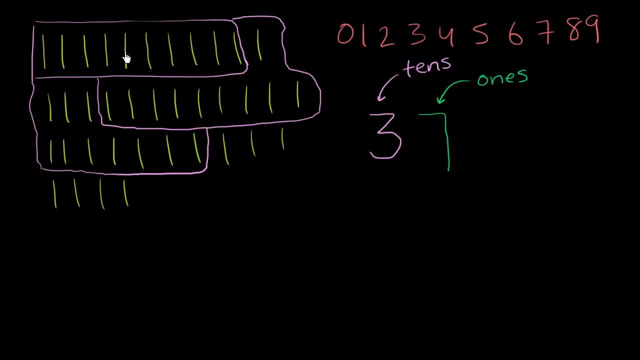 So this essentially tells us the exact same thing. This tells us the exact same thing, The exact same thing as this does right over here. This tells us three 10s: One, two, three, Three 10s, Three groups of 10.. 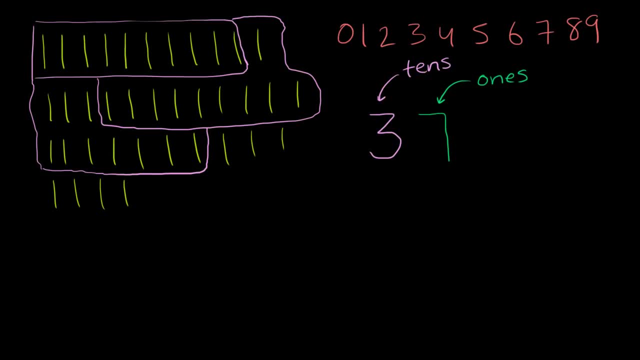 And then another seven ones. So we could rewrite this: This is equal to three 10s plus seven ones, Or another way to think about it. what are three 10s? Well, if we use the same number system to represent three 10s, 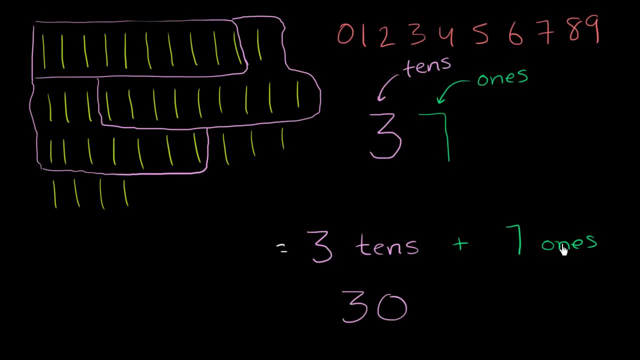 you would write that down as 30. And then seven ones once again. if you use our same number system, you would represent that as seven. So these are all different ways of representing 37. And hopefully this allows you to appreciate how neat our number system is.